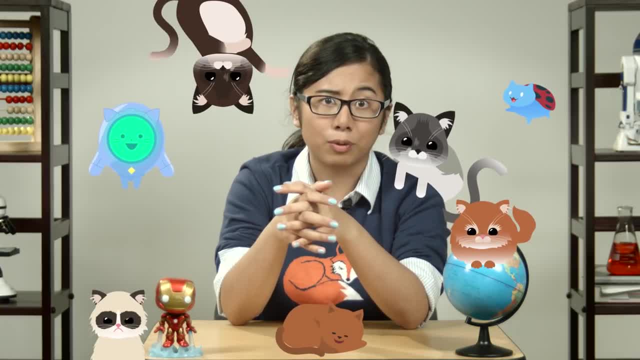 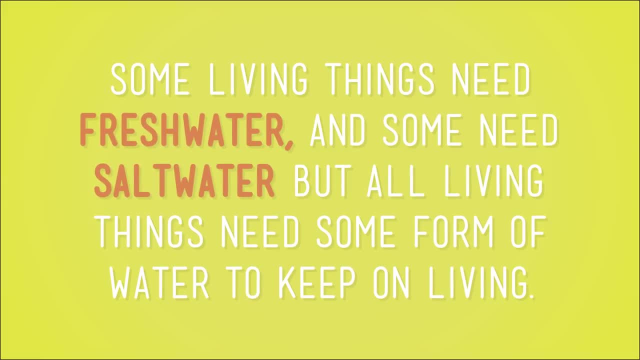 No, not YouTube videos of cats, although it's hard to imagine life without them. I'm talking about water. Living things need water. Some living things need fresh water and some need salt water, But all living things need some form of water to keep on living. 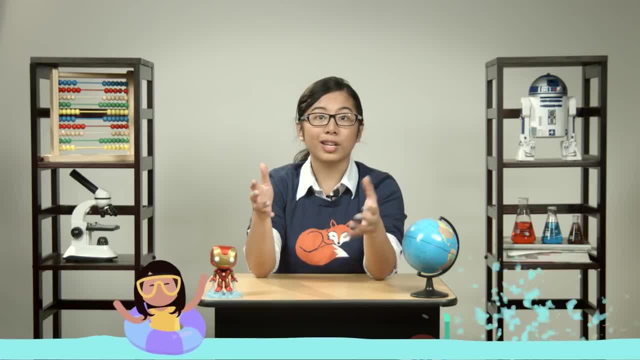 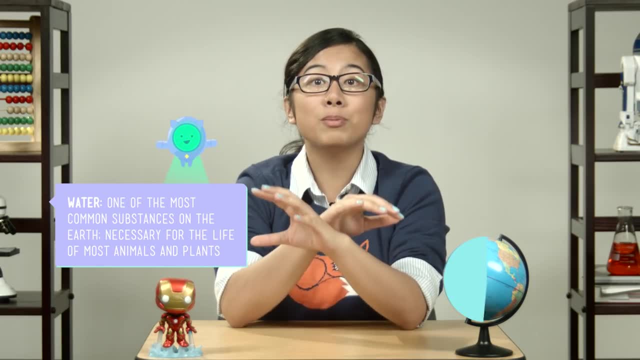 I know you know what water is, You've seen it, you've done cannonballs into it, you've filled balloons with it and threw them at people, And you certainly drink it. Water is one of the most common substances on Earth. It covers more than two-thirds of the surface of our planet. 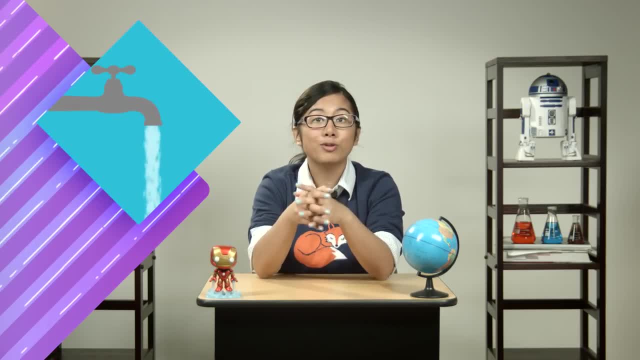 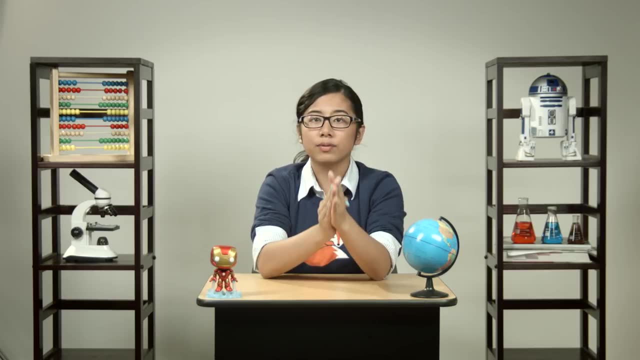 We actually have enough water on Earth to leave a faucet running for 136 trillion years, But let's not do that, Because, for all the water we have, there's one kind of water that we need to keep us alive, And that's fresh water. 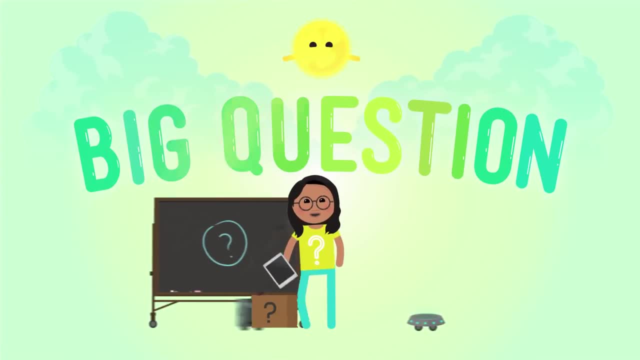 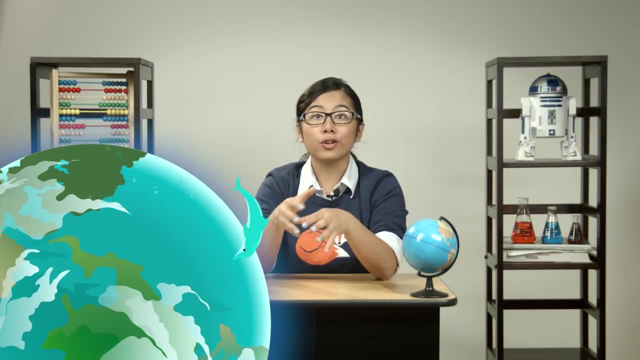 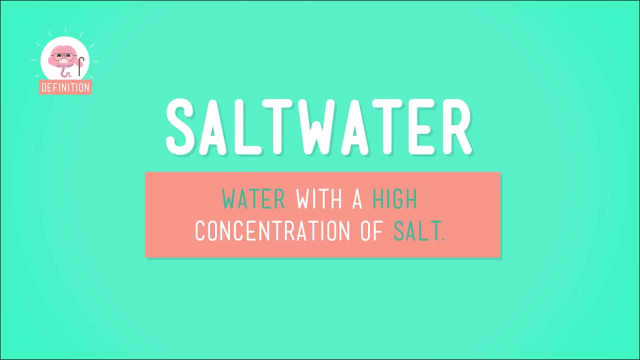 So what is fresh water and where do we get it? Well, it's probably easier to start with where it's not. Most of the water on Earth is in the oceans. They're huge and they're also full of salt, So most of the water on Earth is actually salt water. 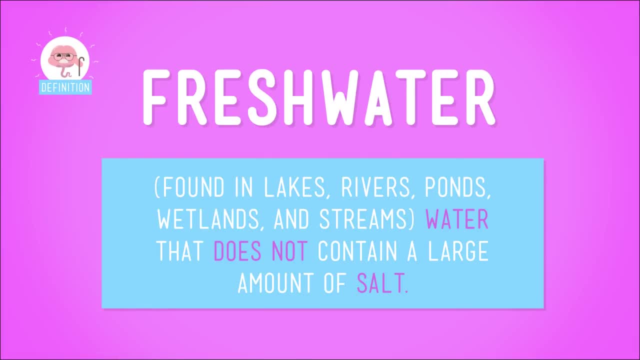 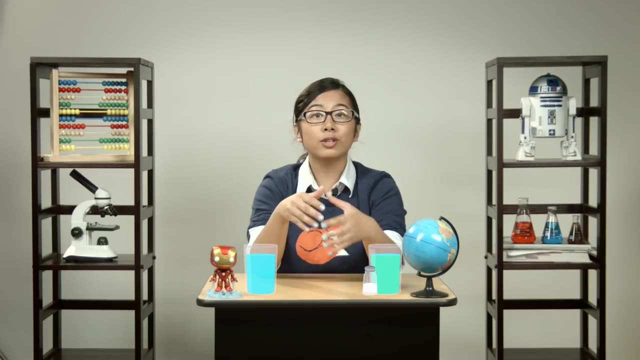 By contrast, fresh water is found in lakes, rivers, ponds, wetlands and streams, and it contains very little salt- Less than 0.1% salt actually- And plants and animals, including us humans, depend on fresh water. 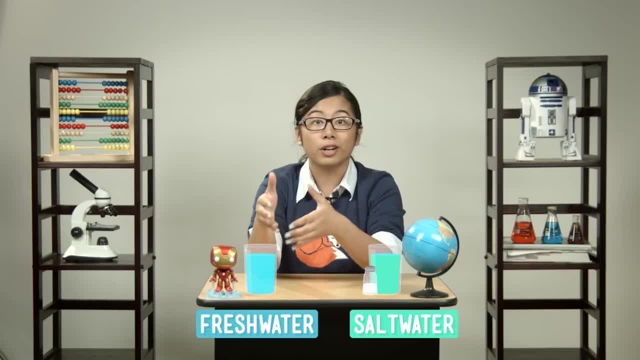 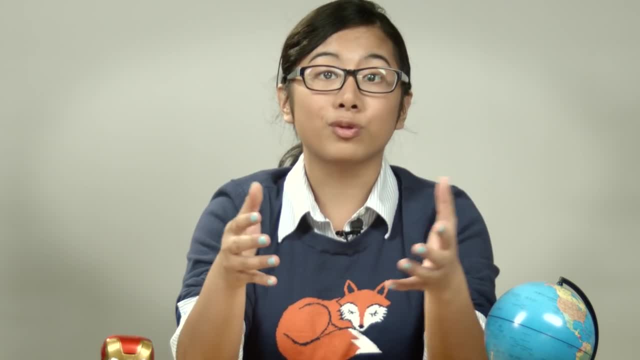 because we can't survive on salt water. The amount of salt in salt water is much higher than what our bodies can process. In fact, drinking too much salt water could even kill a person, which is just one of the reasons fresh water is so important. 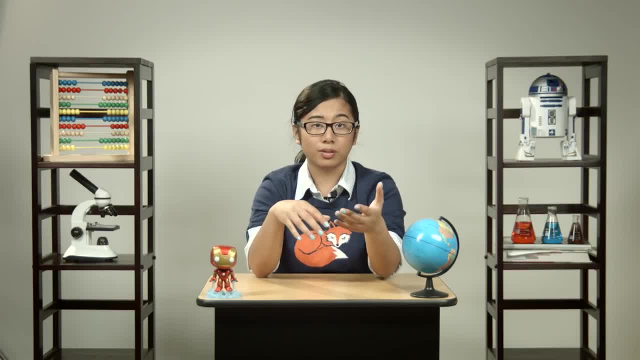 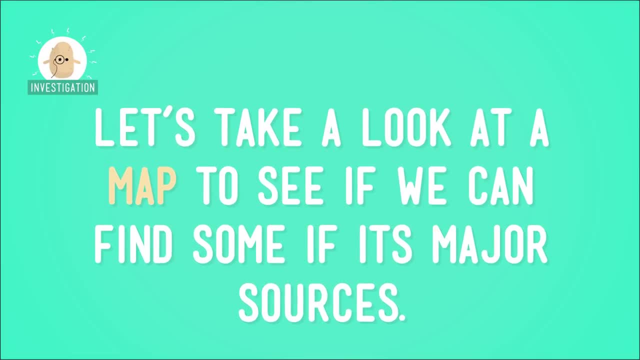 So now you know what fresh water is and that it's super necessary to our survival. But if the oceans make up most of the water on Earth, where can you find fresh water? Let's take a look at a map to see if we can find some of its major sources. 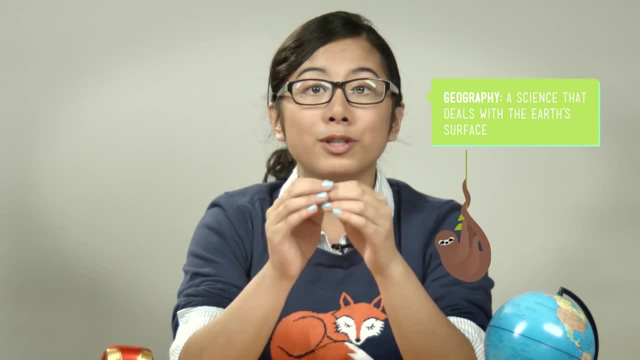 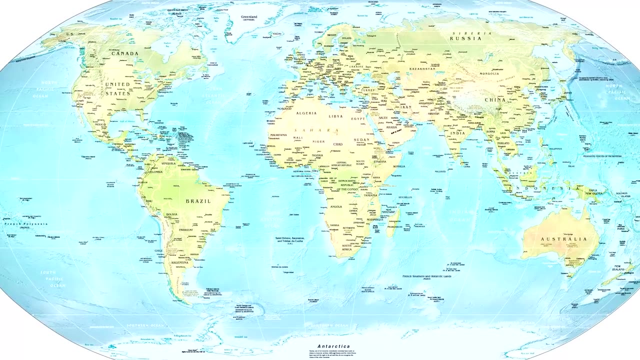 People who study geography- we call them geographers- use maps all the time. They're interested in Earth's physical features like its mountains, deserts, rivers and oceans. This map shows all of the Earth's land and water. All of the blue stuff is water. 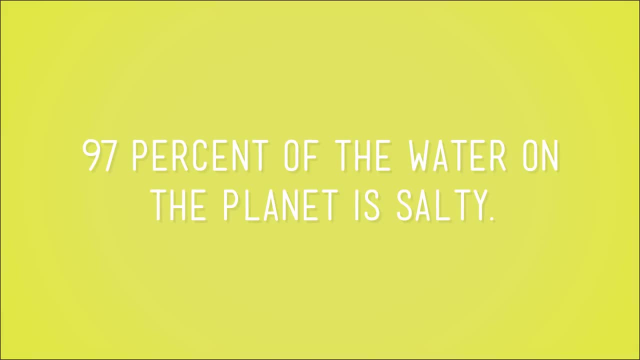 But remember, most of the blue stuff is salt water. In fact, about 97% of the water on the planet is salty. So if you want to know what salt water is, you need to know what salt water is. So if you want to know what salt water is, you need to know what salt water is. 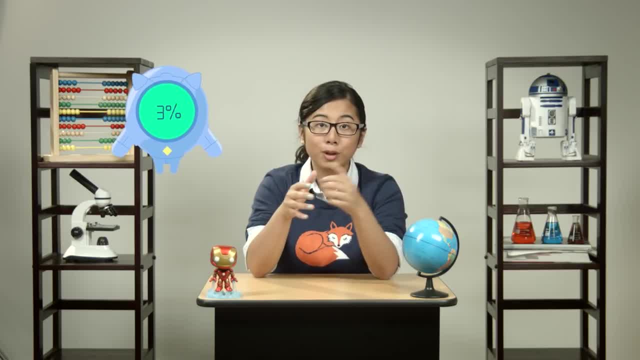 So if you want to know what salt water is, you need to know what salt water is. So let's do some math with that. If 97% of the Earth's water is salt water, then only about 3% of the planet's total water supply is fresh water. But about 2% is locked up in frozen glaciers or underground where we can't get to it. So that means of all the water that's on Earth, less than 1% of it is actually accessible to us on the surface.